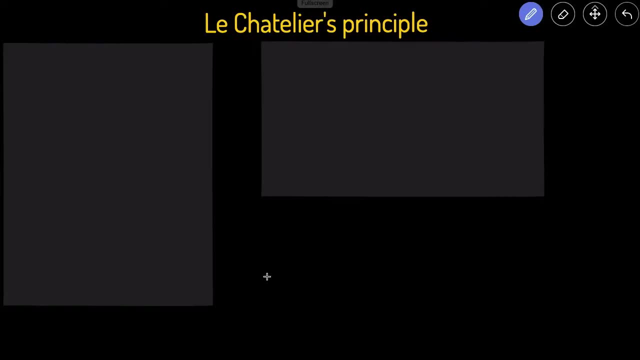 Hey guys, Michael from Concord Chemistry, In this video we'll be talking about Le Chatelier's principle, What it is, how it can help you determine which way the reaction will shift, and we'll be going through several problems together. The setup for Le Chatelier's principle: 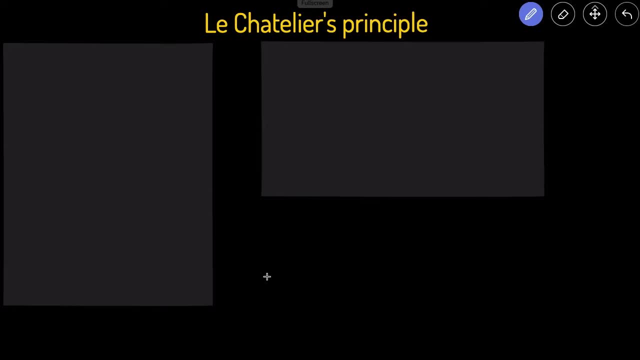 is you currently have a reaction that is at equilibrium, Then some stress, some change occurs that kicks the system out of equilibrium. This principle can help you determine which way the reaction will shift- towards the product or towards the reactants, to re-establish equilibrium. So the 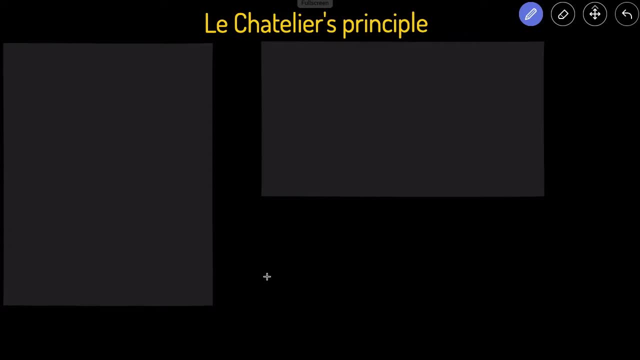 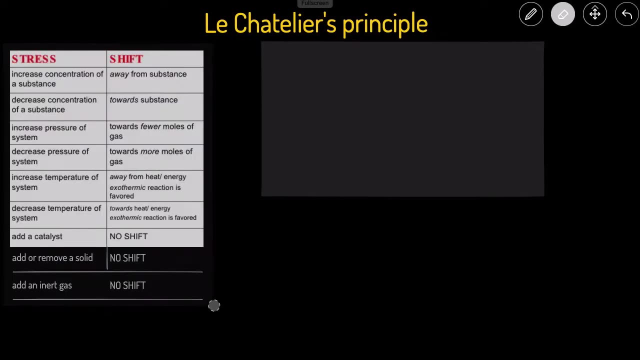 main concept is: it's out of equilibrium. how can I get back to equilibrium? The way the reaction will shift will depend on the type of stress that is induced, And here I have a list of stresses and the guideline in terms of which way the reaction will shift. There's a lot here. I think it's. 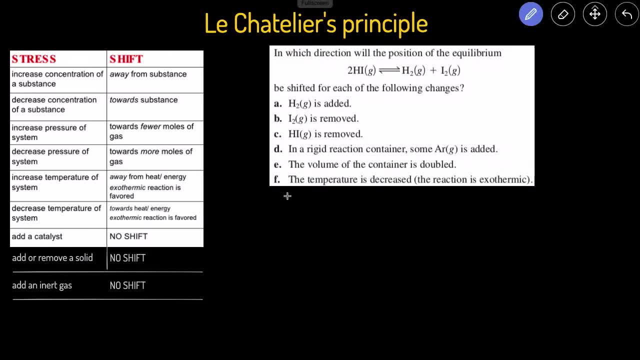 probably easier to just take a look at the example problem and see how that applies. So this question reads: in which direction will the position of the equilibrium of this balanced chemical reaction be shifted when each of these changes occur? So the first part A is we're adding H2.. 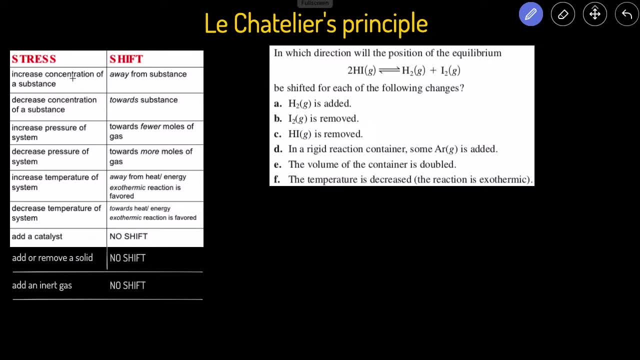 If we're adding H2, you can see that whenever we increase the concentration of something, it shifts away from that side. So if we add some H2, and since H2 is on the product side, the reaction will shift to the left. so go to the reactant side. 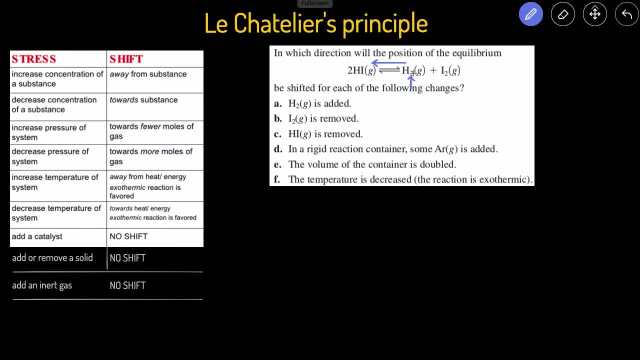 Why is that? It's because we wanna offset the change. If we're adding more products, then we're going to want to shift away from the product side to get rid of some of those products and to make more reactants. So the answer for part A. 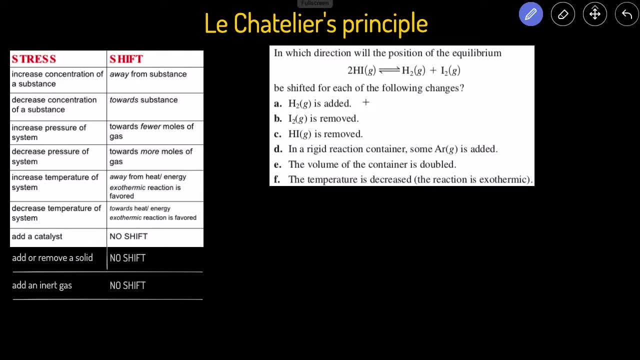 is that the reaction will shift to the left. Part B, I2 gas, is removed. That would be decreasing the concentration of the I2.. Whenever you decrease the concentration of the substance, it will move towards the side that contains the substance. So, since we're decreasing the amount of I2,, 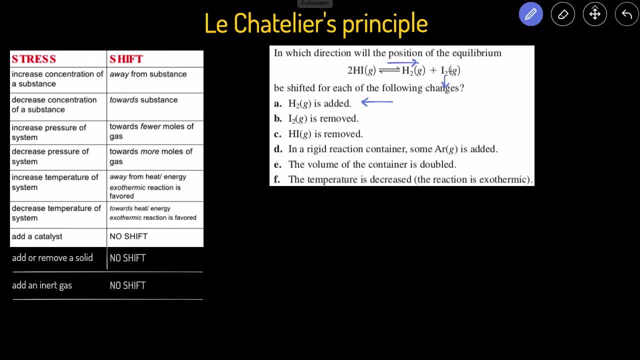 is going to shift to the right to make up to make some more i2. so the answer for part b is that the reaction will shift towards the product side to increase the amount of products and to decrease the amount of reactants. part c, h i gas is removed. so once again we're removing a substance and this 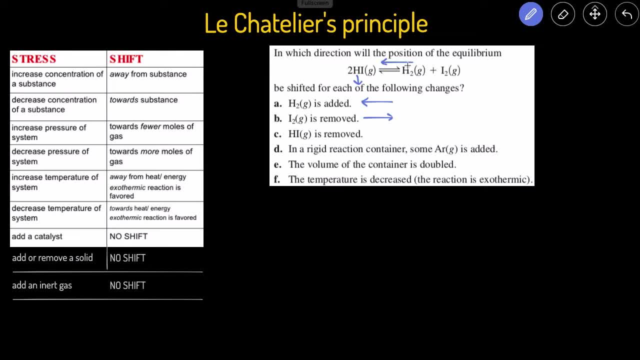 time we're removing the reactants, which means that the reaction will shift towards the reactants, because whenever you remove something it'll shift to that side, so it'll be going to the left shift. part d: in a rigid container, some argon gas is added. that falls under the category of adding. 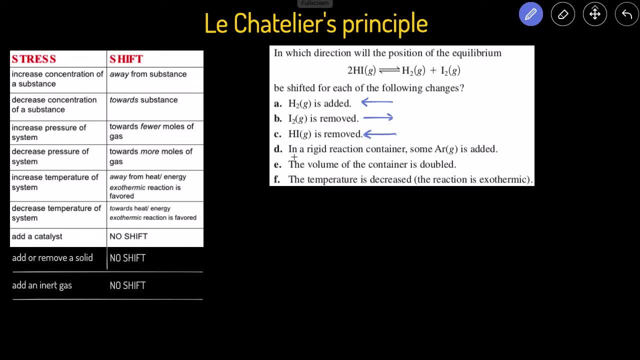 an inert gas. inert just means the gas is unreactive. we know that argon is noble gas. so if we add argon that's not going to affect the amount of hi, h2 or i2, because argon is not going to react of any of. 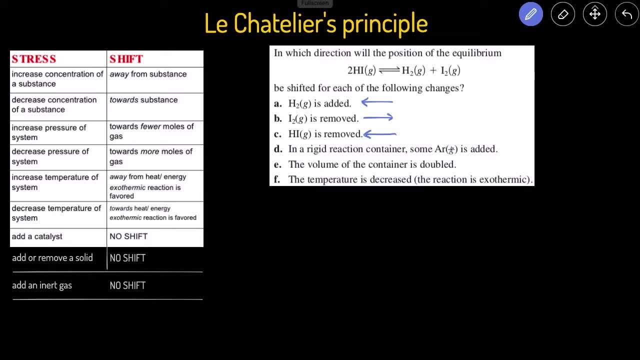 them. so since there we're adding a noble gas and it's not affecting the reaction products, there's going to be no shift here. the reaction is just going to stay at equilibrium part e. the volume of the container is doubled. so when, when you double, when you increase the volume of a container, 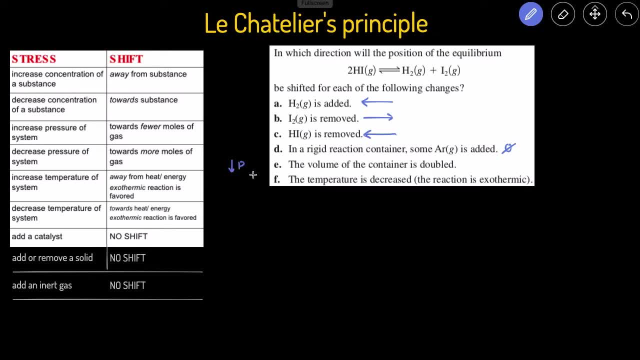 you're essentially decreasing the pressure. so what we're doing in part e is we're decreasing the total pressure of the system, and when we decrease the pressure of a system, the reaction is going to want to move towards the side, with more moles of gas to re-increase the pressure, and so we have. 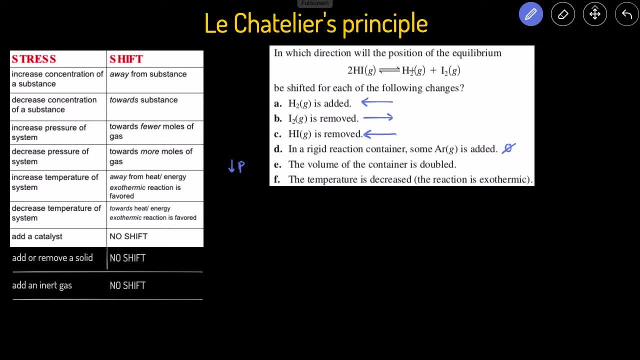 two moles of gas on the left because of coefficient of two here, and then we also have two more moles of gas on the right because we have one plus one. so since there's equal number of moles of gas on both sides, there's not going to be any shifts. if there happened to be a coefficient of 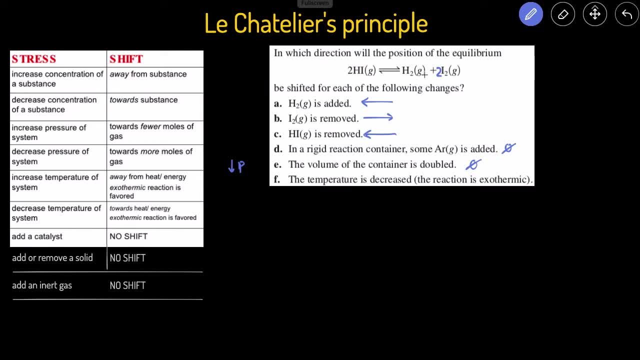 two. here we'll have two moles on the left and then three moles on the right. then the reaction shift to the right because there's more moles of gas on the right than the left, f the temperature is decreased and it tells us that the reaction is exodermic. it's important to know whether the 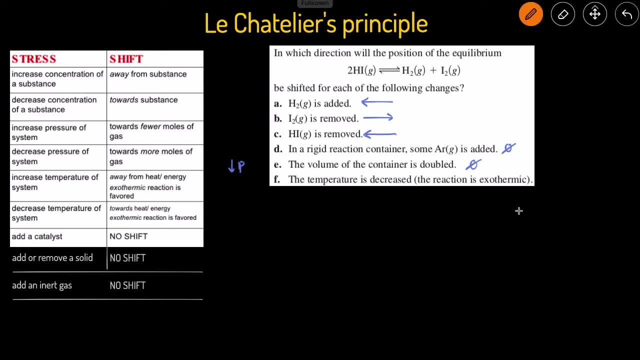 reaction endodermic or exodermic, because that will determine how the reaction will shift when temperature changes. so if a reaction is exodermic, then that means heat is on the product side, because heat is being released, and if the reaction is endodermic it means that 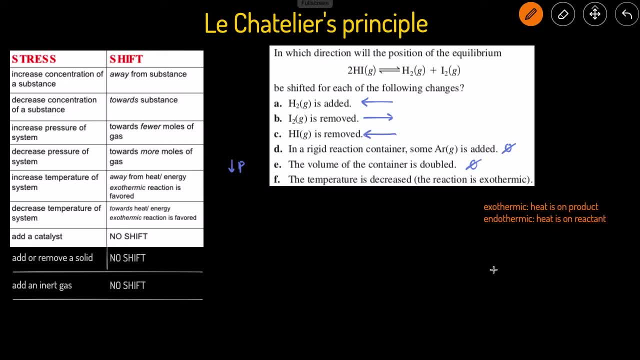 heat is being absorbed. so heat is on the reacting side. it tells us this: this reaction is exodermic, so we can go ahead and add heat on the product side and it says that the temperature is decreased. you can think of decreasing the temperature. is the?